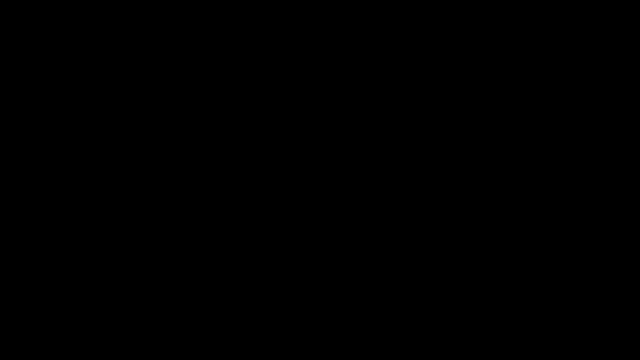 Most of what we do early on, when we first learn about calculus, is to use limits. We use limits to figure out derivatives of functions. In fact, the definition of a derivative uses the notion of a limit. It's the slope around the point as we take the limit of points closer and closer to the point in question. 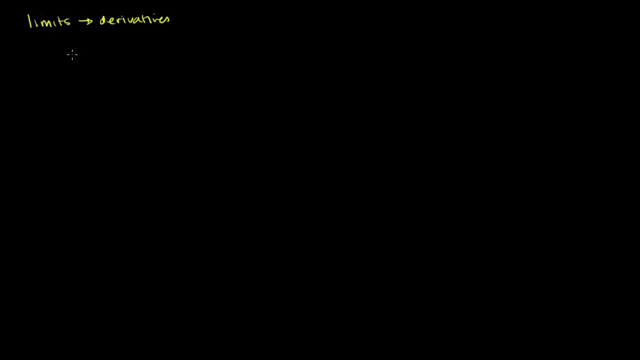 And you've seen that many, many, many times over In this video. we're going to do it in the opposite direction. We're going to use derivatives to figure out limits And, in particular, limits that end up in indeterminate form. 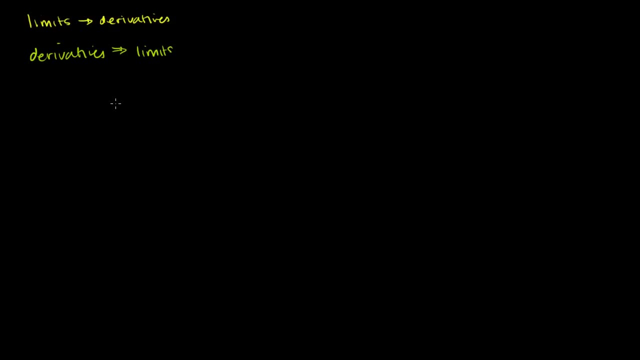 And when I say by indeterminate form, I mean that when we just take the limit as it is, we end up with something like 0 over 0, or infinity over infinity, or negative infinity over infinity, or maybe negative infinity over infinity. 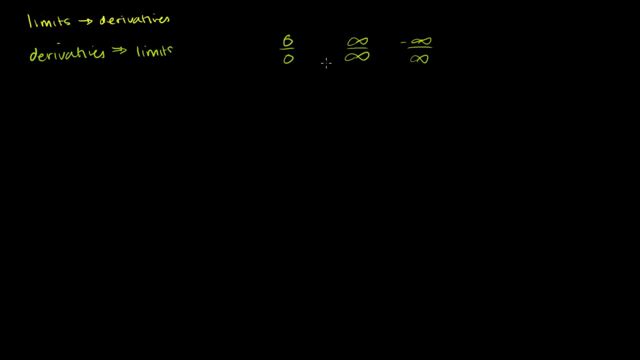 Or positive infinity over negative infinity. All of these are indeterminate, undefined forms, And to do that, we're going to use L'Hopital's rule, And in this video, I'm just going to show you what L'Hopital's 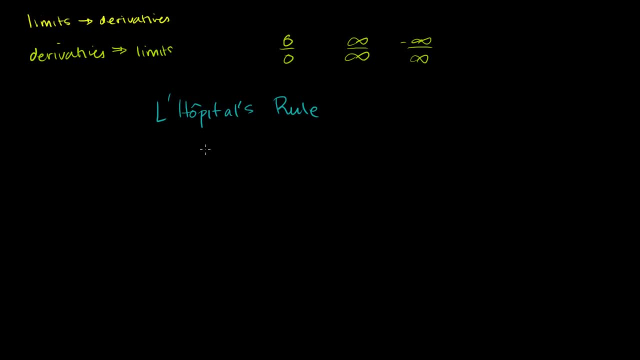 rule says and how to apply it, because it's fairly straightforward and it's actually a very useful tool sometimes if you're in some type of a math company And they ask you to find a hard, a difficult limit that when you just plug the numbers in, you get something like this: 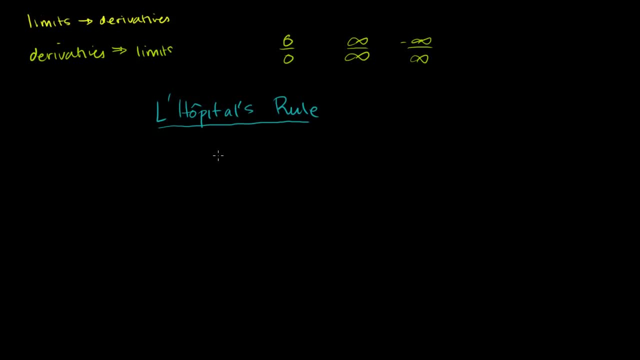 L'Hopital's rule is normally what they are testing you for, And in a future video I might prove it, but that gets a little bit more involved. The application is actually reasonably straightforward, So what? L'Hopital's rule tells us that if we have- and I'll 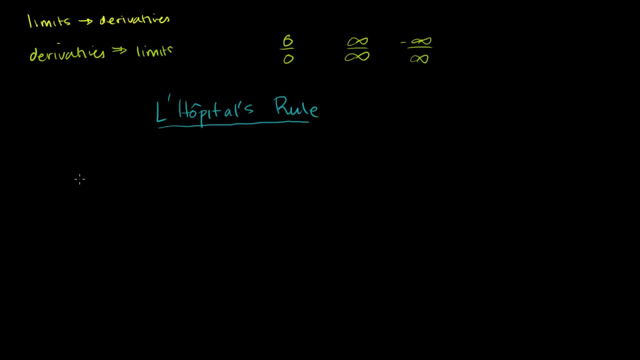 do it in abstract form first, but I think when I show you the example, it will all be made clear that if the limit, if the limit as x approaches c, of f, of x is equal to 0, which is also so if this is equal to 0, and the limit as x approaches c, 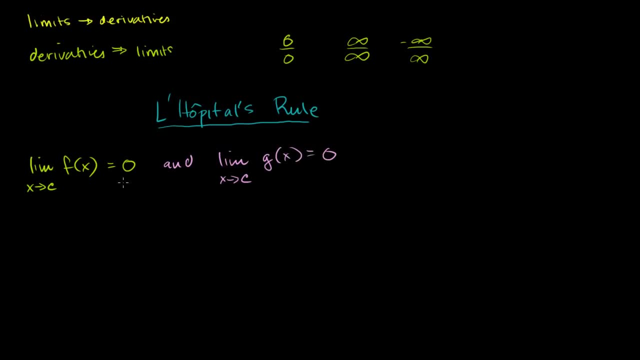 of g of x is equal to 0, and, and this is another and and the limit, the limit as x approaches c, of f prime of x over g prime of x exists and it equals L, then. so all of these, 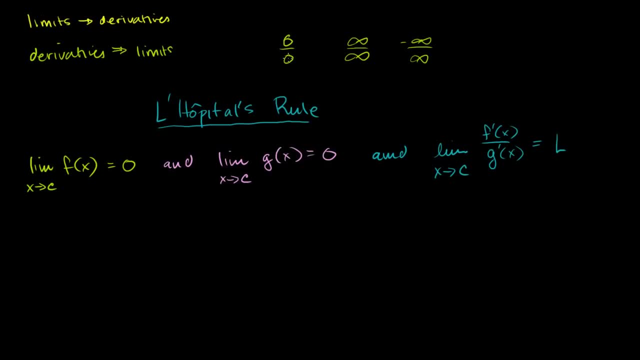 conditions have to be met. This is the indeterminate form of 0 over 0, so this is the first case. Then then we can say that the limit, as x approaches c of f of x over g of x, is also going to be equal to L. 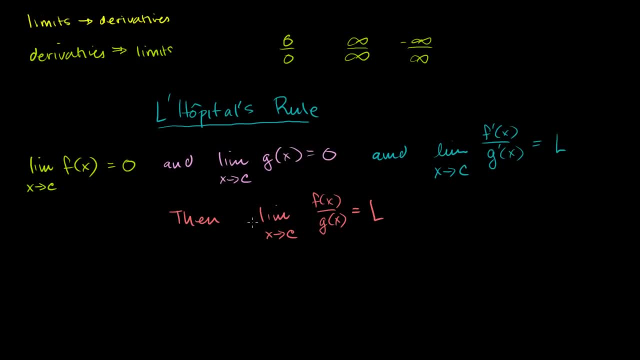 So this might seem a little bit bizarre to you right now, and I'm actually going to write the other case and then I'll do an example, and we'll do multiple examples and the examples are going to make it all clear. So this is the first case and the example we're going to do. 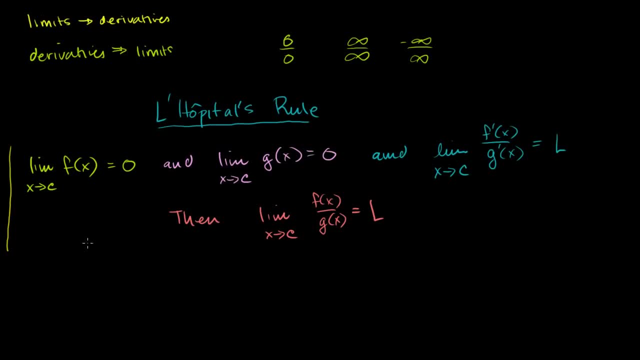 is actually going to be An example of this case. Now, the other case is if the limit as x approaches c of f of x is equal to positive or negative infinity And the limit as x approaches c of g of x is equal to positive, 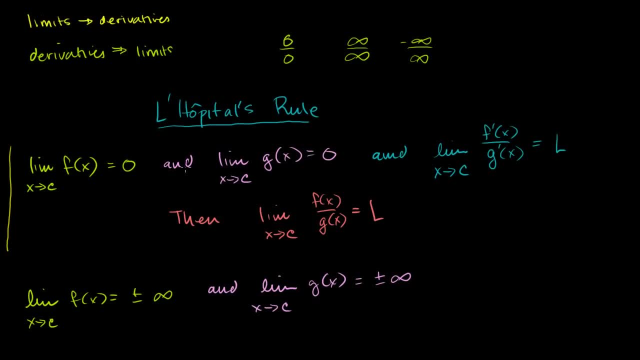 or negative infinity, And And And And, And. the limit of, I guess you could say the quotient of the derivatives, exists And the limit, as x approaches c of f prime of x over g prime of x is equal to l. 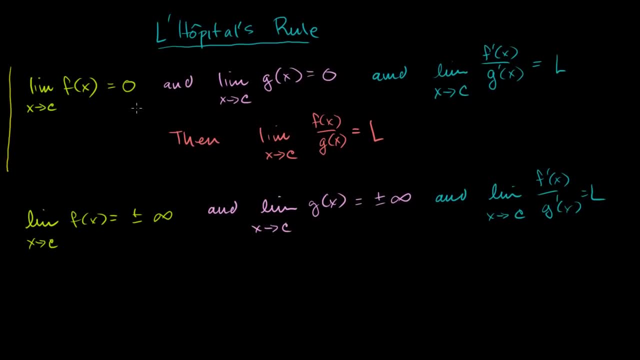 Then we can make this same statement again, Then we can make this exact statement again. Let me just copy that out, Then this again Edit copy, and then let me paste it. So in either of these two situations, and just to kind of make sure you understand what you're looking at- 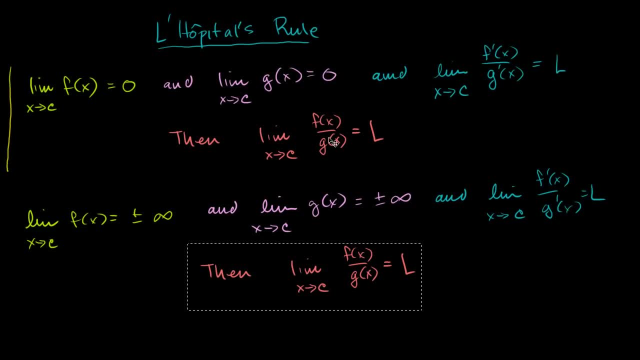 this is a situation where, if you just tried to evaluate this limit right here, you're going to get f of c, which is 0, or the limit as x approaches c of f of x, over the limit as x approaches c of g of x, and that's going to give you 0 over 0.. 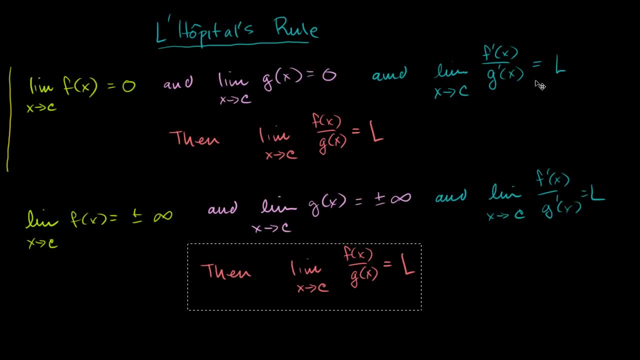 And so you say, hey, I don't know what that limit is. But this says: well, look, if this limit exists, I could take the derivative of each of these functions and then try to evaluate. I could take that limit and if I get a number, if that exists, then they're going to be the same limit. 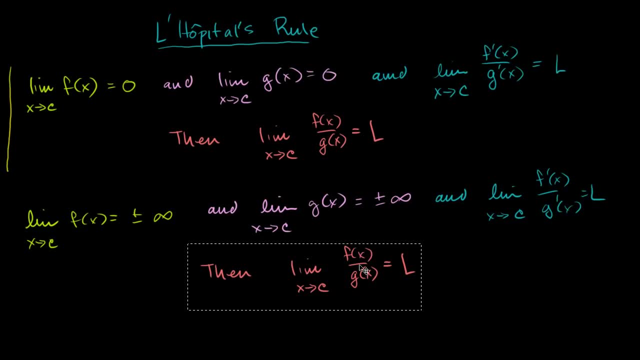 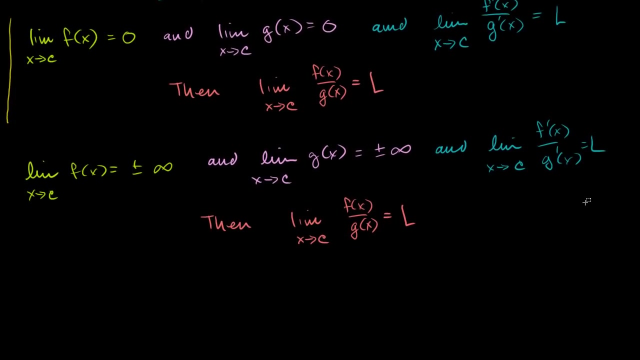 This is a situation where, when we take the limit, we get infinity over infinity or negative infinity, or positive infinity over positive or negative infinity. So these are the two indeterminate forms And to make it all clear, let me just show you an example, because I think this will make things a lot more clear. 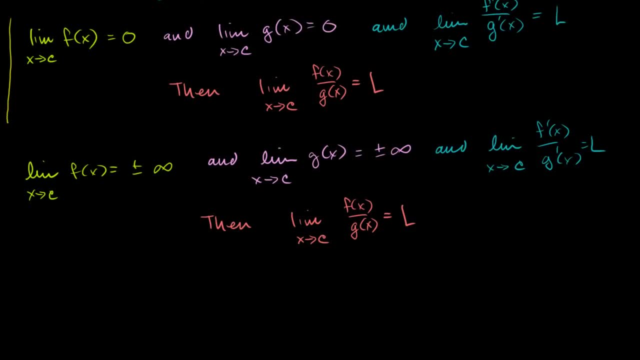 So let's say we are trying to find the limit. Let me do it in this purplish color. Let's say we wanted to find the limit as x approaches 0, of sine of x over x. Now, if we just view this, if we just try to evaluate it at 0,, 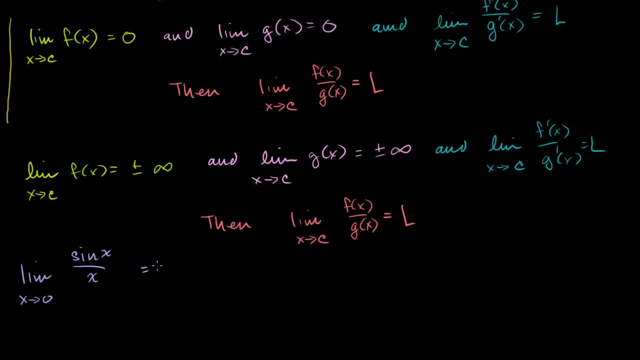 or take the limit as we approach 0. in each of these functions we're going to get something that looks like 0 over 0.. Sine of 0 is 0.. Or the limit as x approaches 0 of sine of x is 0. 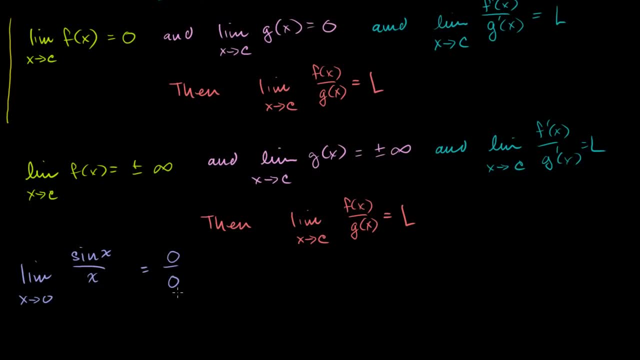 And obviously, as x approaches 0 of x, that's also going to be 0. So this is our indeterminate form And if you want to think about it, this is our f of x. That f of x, right, there is sine of x. 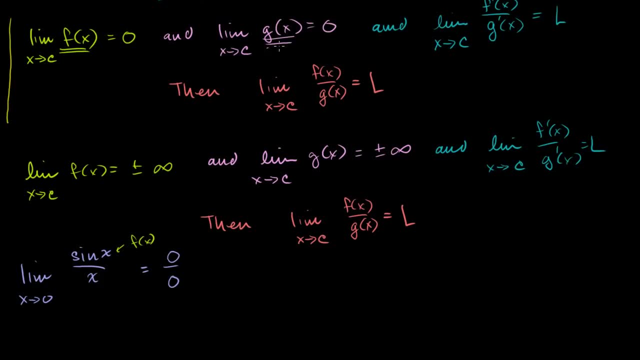 And our g of x. this g of x right there for this first case is the x Right. g of x is equal to x And f of x is equal to sine of x. And notice, Well, we definitely know. 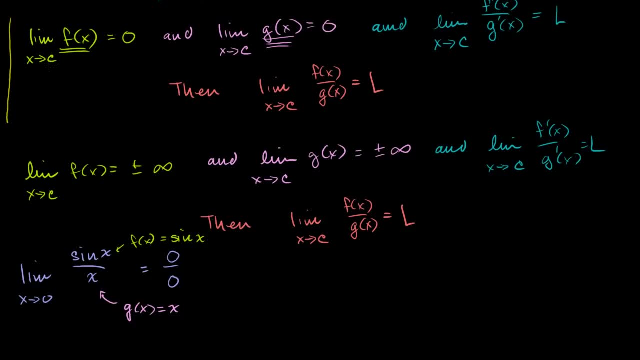 That this meets the first two constraints. The limit as x, and in this case c, is 0.. The limit as x approaches 0 of sine of x is 0.. And the limit as x approaches 0 of x is also equal to 0. 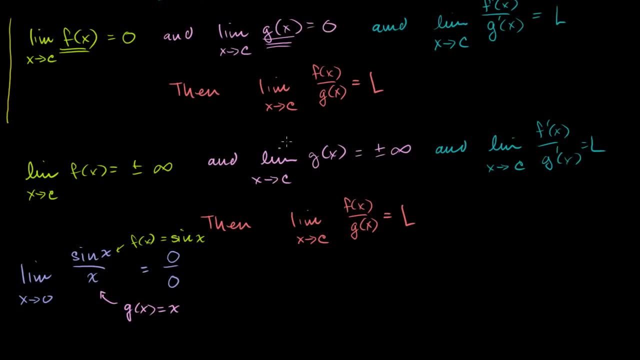 So we get our indeterminate form. So let's see at least whether this limit even exists If we take the derivative of f of x and we put that over the derivative of g of x and take that limit as x approaches 0, in this case. 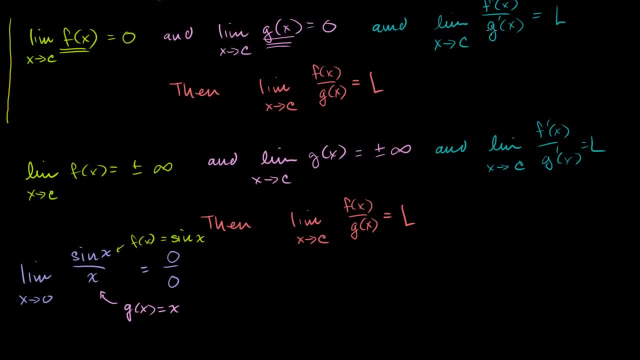 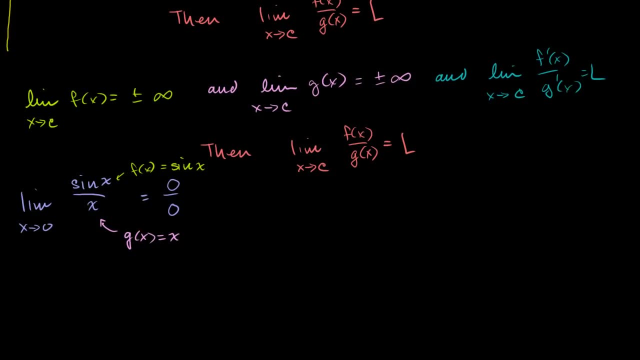 x approaches 0, that's our c. Let's see if this limit exists. So I'll do that in the blue. So let me write the derivatives of the two functions. So f- prime of x. If f of x is sine of x, what's f? prime of x? 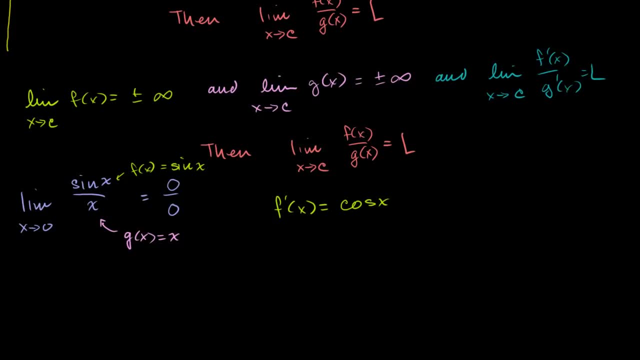 Well, it's just cosine of x. We've learned that many times. And if g of x is x, what is g, prime of x? That's super easy: The derivative of x is just 1.. So let's see, Let's try to take the limit. 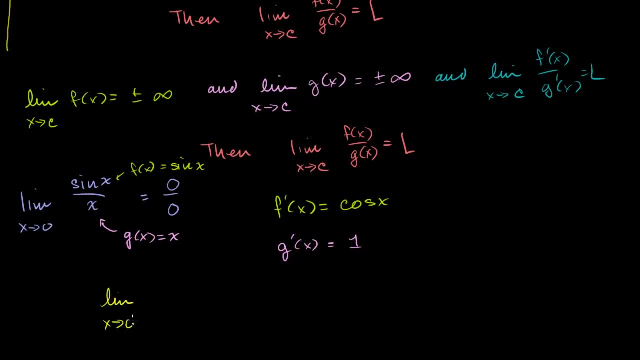 Let's try to take the limit as x approaches 0 of f prime of x over g prime of x over their derivatives. So that's going to be the limit as x approaches 0 of cosine of x over 1.. I wrote that 1 a little strange. 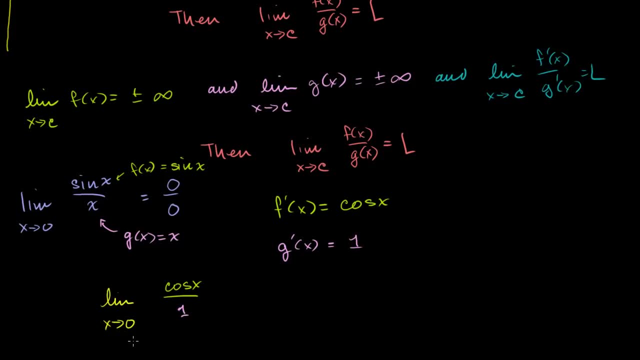 Over 1.. And this is pretty straightforward. What is this going to be? Well, as x approaches 0 of cosine of x, that's going to be equal to 1.. That's equal to 1.. And obviously, the limit as x approaches 0 of 1,. 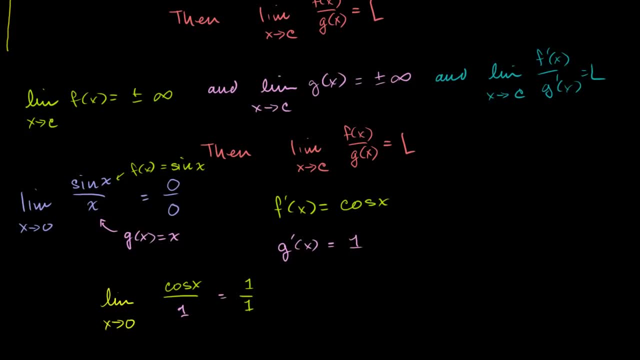 that's also going to be equal to 1.. So in this situation, we just saw that the limit as x approaches our c, in this case, is 0,. as x approaches 0 of f, prime of x over g prime of x is equal to 1.. 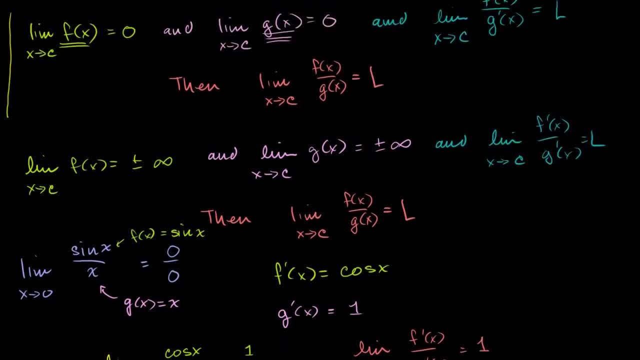 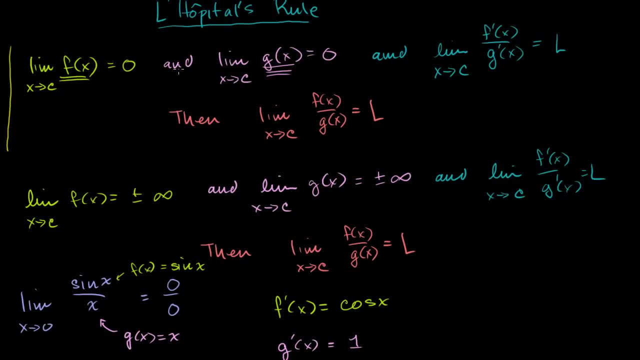 This limit exists and it equals 1.. So we've met all of the conditions. This is the case we're dealing with. Limit as x approaches 0 of sine of x is equal to 0.. Limit as x approaches 0 of x is also equal to 0. 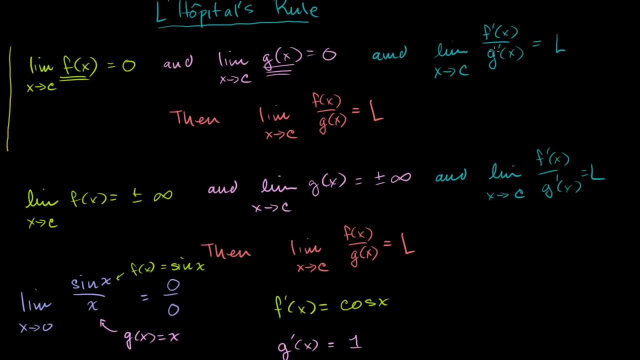 The limit of the derivative of sine of x over the derivative of x, which is cosine of x over 1, we found this to be equal to 1.. So all of these top conditions are met. So then, we know this must be the case. 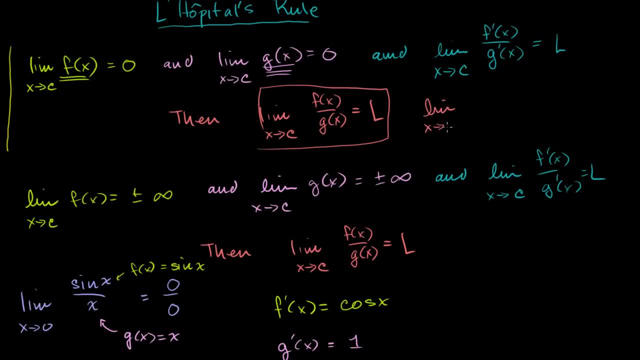 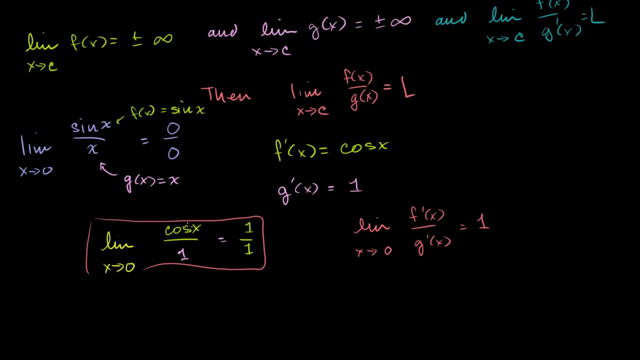 that the limit, as x approaches 0, of sine of x over x must be equal to 1.. It must be the same limit as this value right here where we take the derivative of the f of x and of the g of x. I'll do more examples in the next few videos.